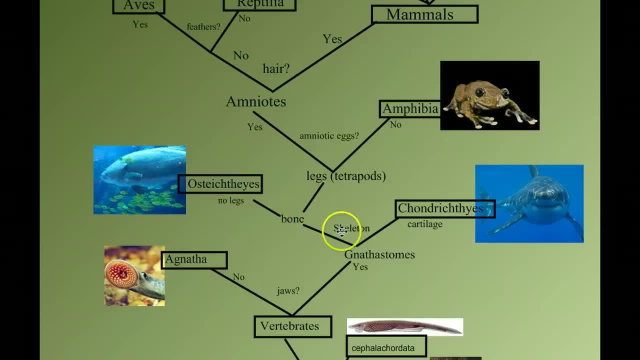 we're going down this branch of those vertebrates with a bony skeleton that have legs, or are tetrapods, four limbs Within the tetrapods, those vertebrates with limbs, we have to ask the question: do we have an amniotic egg, Yes or no, When we go down the no branch? 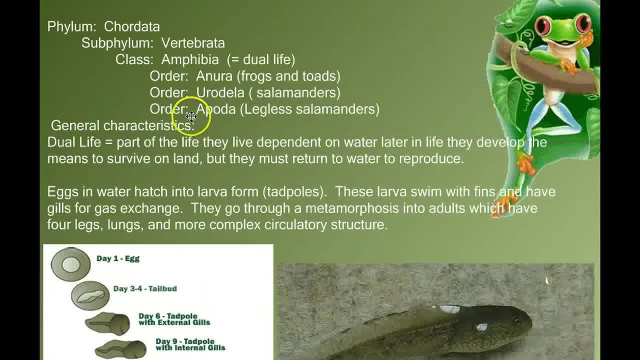 we get to the class Amphibia, The first thing we need to do is look at what the word amphibia means. Amphi means dual Bia, bios. bio means life, Dual life. Now think about what you know about amphibians and see if that makes sense. 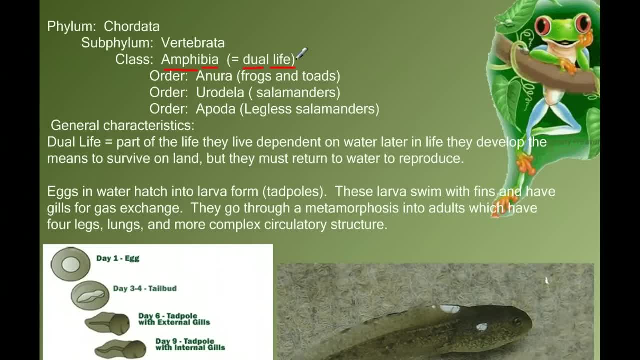 The defining characteristic of this class of animal is that they live part of their life in water, dependent on water, and part of their life on land. These are the frogs and toads, the salamanders and the legless salamanders In this class. I'm going to ask: 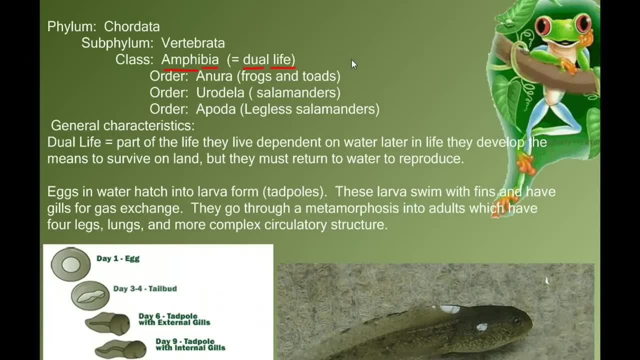 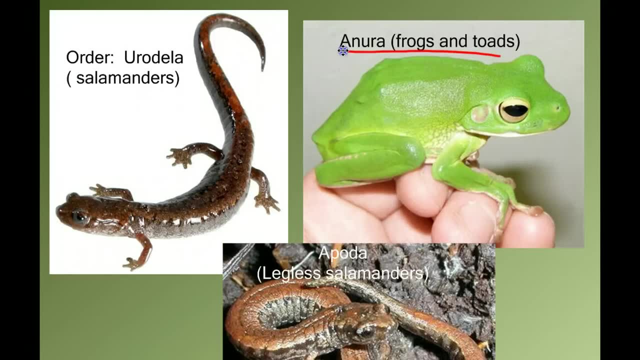 you to know the specific orders, or these three orders: The order Anura for the frogs and toads, the order Urodela for the salamanders and the order Anura for the frogs and toads. The order Anura for the frogs and toads and the order Urodela for the salamanders. 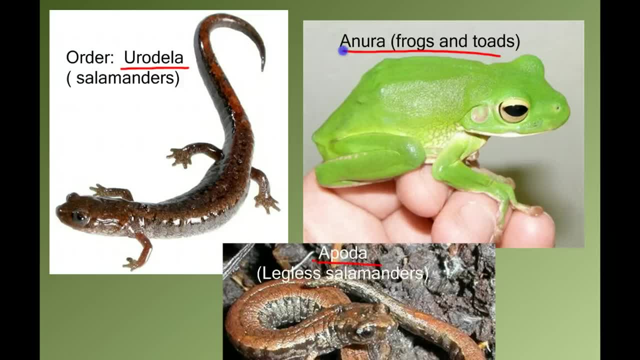 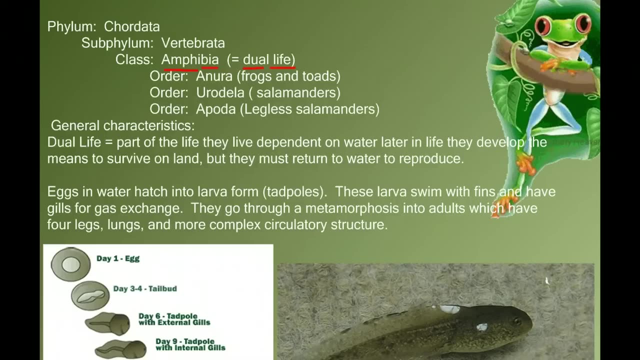 and the order Apoda for the legless salamanders. A lacking poda, pods, legs, appendages, legless, the legless salamanders. Now, the biggest thing for us here is that the amphibians represent for us a transition. 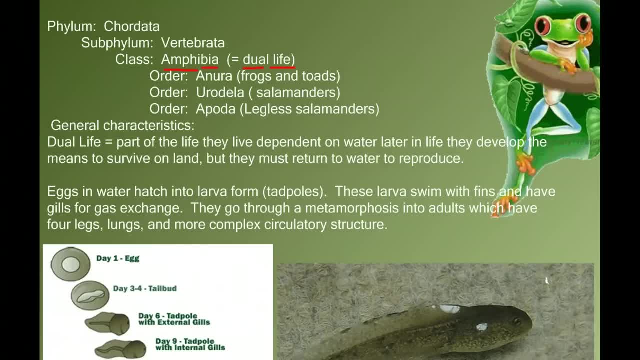 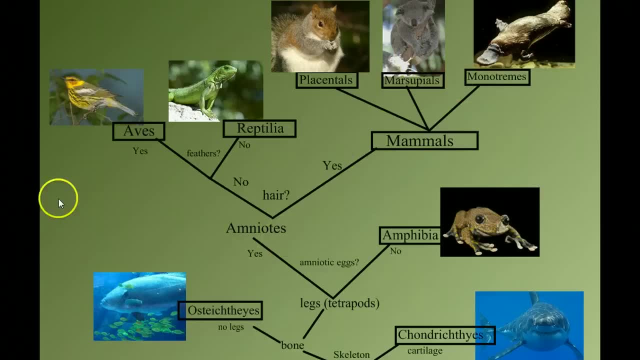 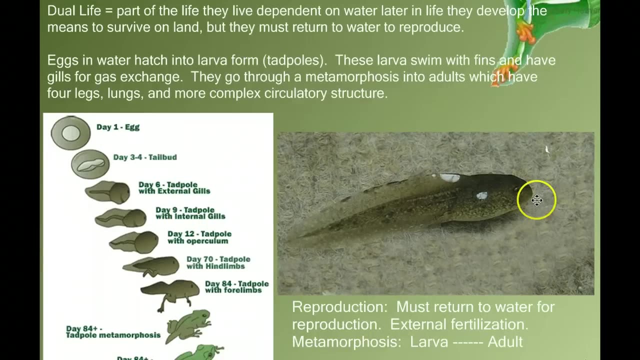 Not only do amphibians go through a transition from water to land, but for us they represent the transition from the fish to the terrestrial animals, and they are in between. All amphibians must start their life in water. They are tadpoles. The tadpoles are fish-like in that. 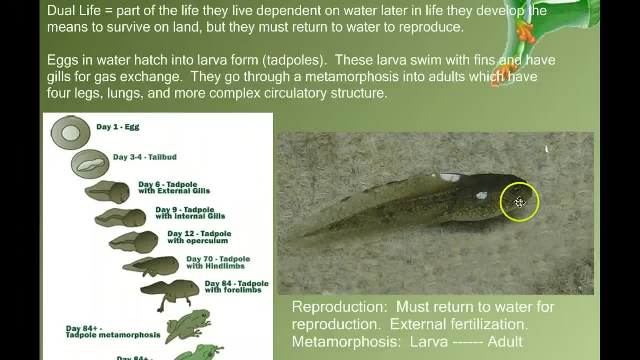 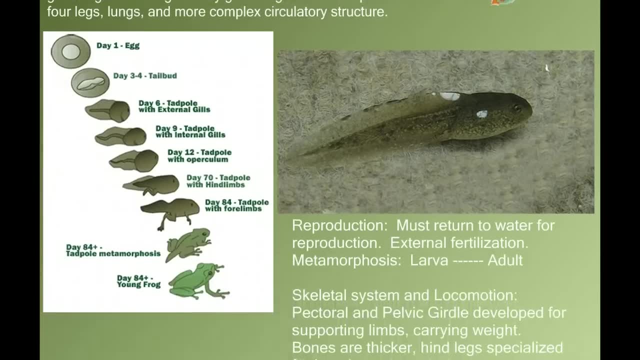 they swim and they have gills and they couldn't exist on land. They don't have limbs, they have fins, so they have to start out in water. But they go through a metamorphosis where they change, growing limbs, reducing a tail- in the frog at least- and developing lungs. 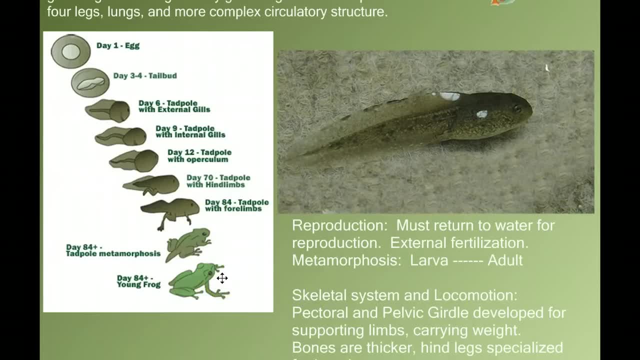 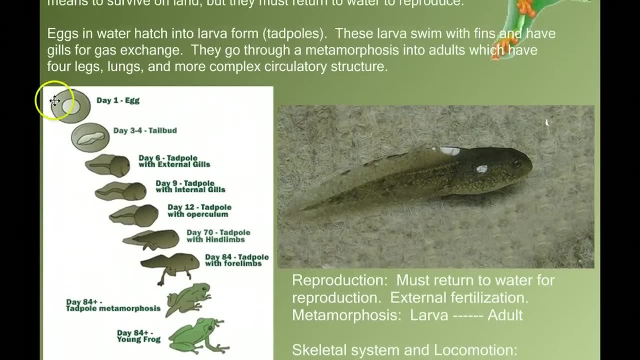 There's also going to be a change in the circulatory system that goes along with this change. So those are all the things we need to investigate: is this transition within one life from water onto land, but also how that represents in the evolutionary sense. 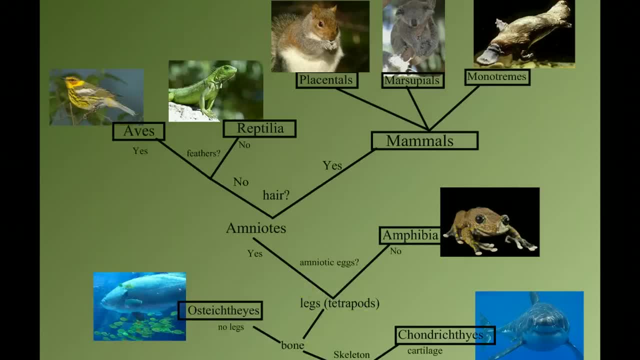 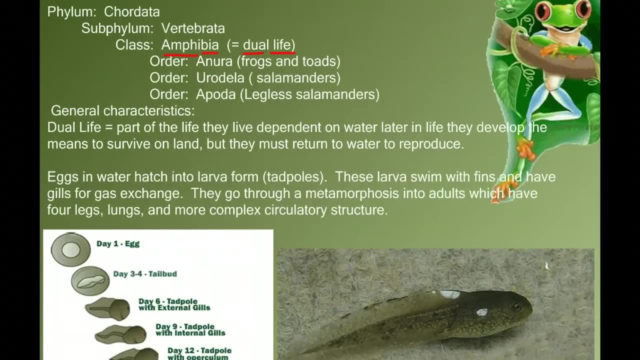 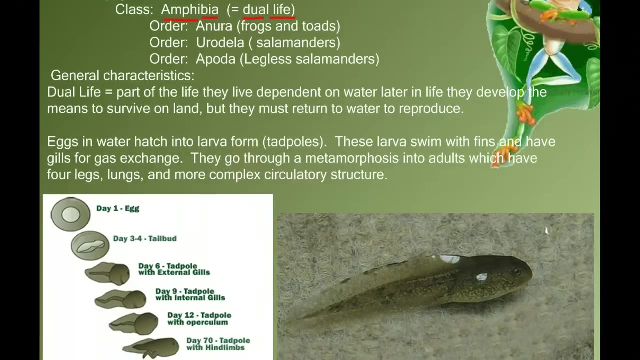 the transition for vertebrates from water onto land. So it's a nice parallel case study for us. So again, the most obvious characteristic of these animals is that they are dependent on water for reproduction. They must reproduce in water. The egg that they lay is not an. 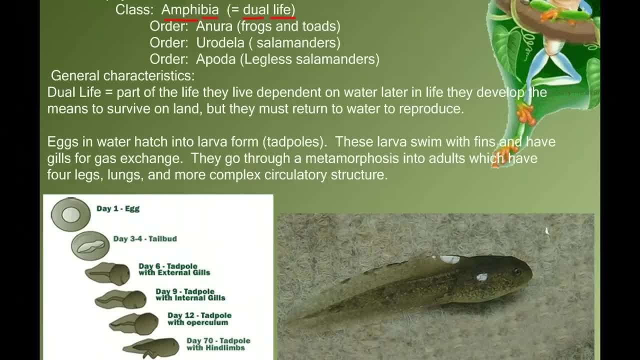 amniotic egg. It cannot survive. It's outside of water. So for the first time in this group, we're going to see limbs and we're going to see lungs and we're going to see a change in the circulatory system as they move from the 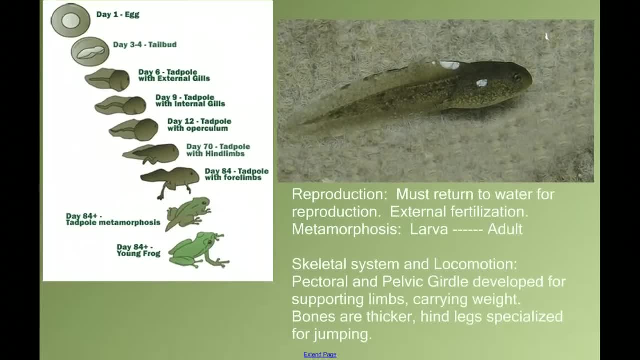 aquatic tadpoles into the adult terrestrial animal Must return to water for reproduction. external fertilization and the metamorphosis is kind of a major characteristic: The skeletal system. when we move onto land, the skeletal system has to become thicker. It's going to support the physical weight of the body, whereas in 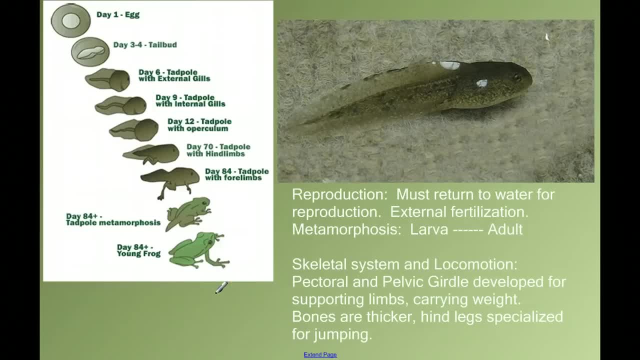 water, the weight is carried by the water itself, Kind of like when we talked about plants moving onto land, the necessity for internal structural support became more important. Here we're going to see the bones of the amphibian, the adult amphibian, being thicker and more. 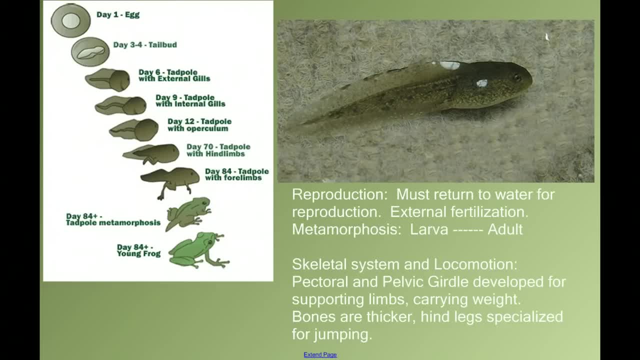 sturdy to carry the weight compared to those of, say, a fish. We're also going to see the development of the pectoral and pelvic girdle to help attach the limbs to the axial spine. While we have these three specific orders, we certainly need to know which ones are which. 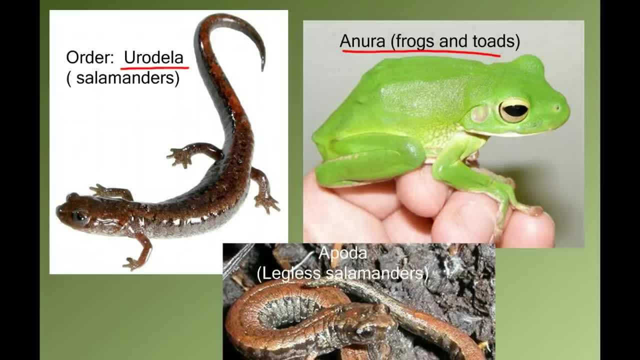 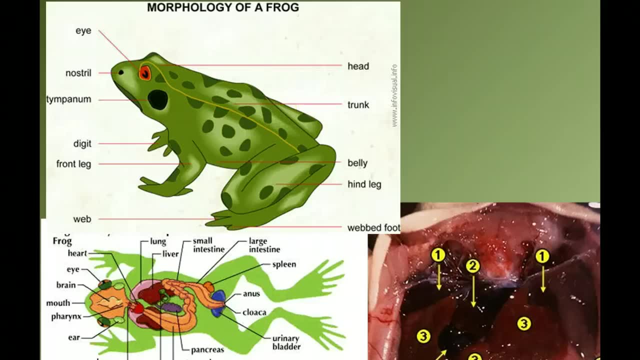 We definitely are going to use the frog, the anura, as kind of the poster child to represent all amphibians for us. We look at the general anatomy of a frog, for example, to run a represent amphibians. We're going to notice a couple of interesting things. First of all, in terms 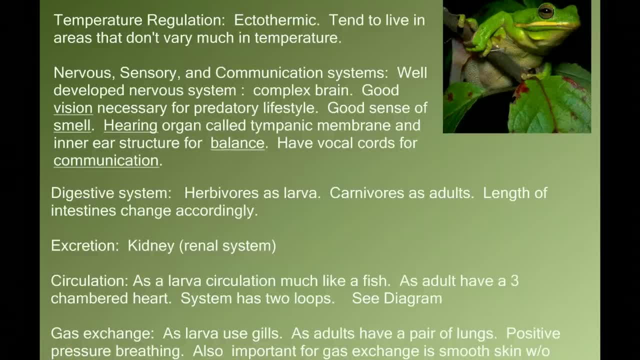 of just characteristics. the amphibians, like fish, are ectotherms, meaning that their temperature depends upon their temperature. We said that with fish this isn't that big of a deal, because their aquatic environment's temperature doesn't change very drastically, or if it does, it doesn't change very fast. 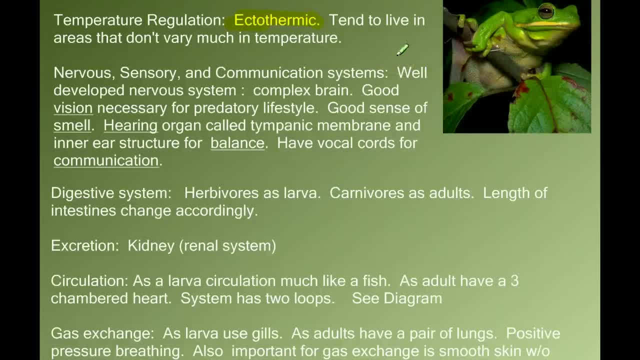 But living on land, air temperatures can change pretty rapidly, and that presents a problem for many amphibians. As a result, they're limited in the habitat that they can inhabit. Those that do live in areas where temperatures can be more extreme- cold or hot- have developed. 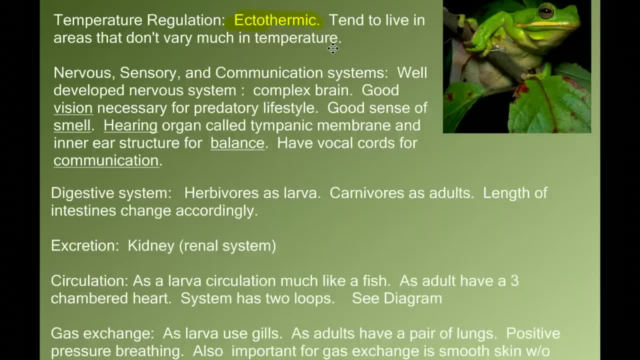 some behavioral techniques to kind of handle that temperature. We know that the amphibians have to develop some sensory and nervous system things that are a little different than being in water. Vision becomes much more important eyesight on land than it is in water. Sense of smell also, But we know that frogs can hear. We. 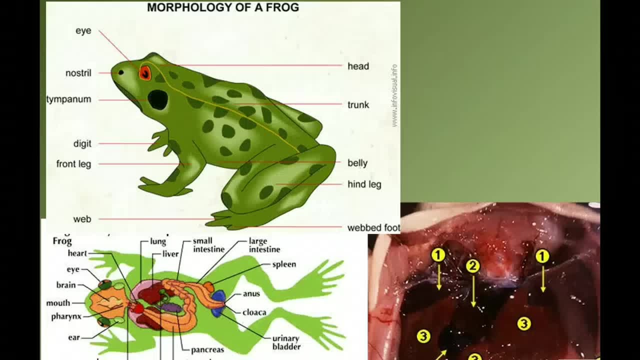 know that frogs can hear because they vocalize. When we look at this diagram of a frog, there's a structure called a tympanum Right here And it's a thin membrane stretched over the opening to the ear canal. They don't. 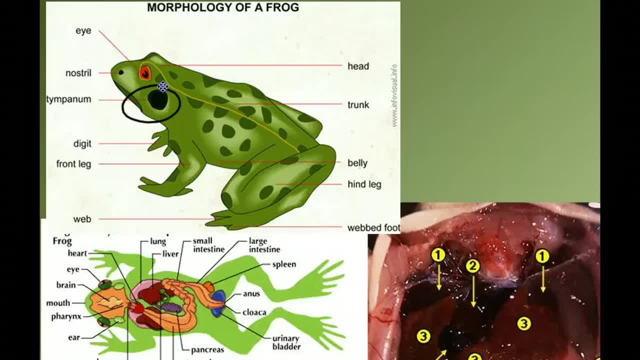 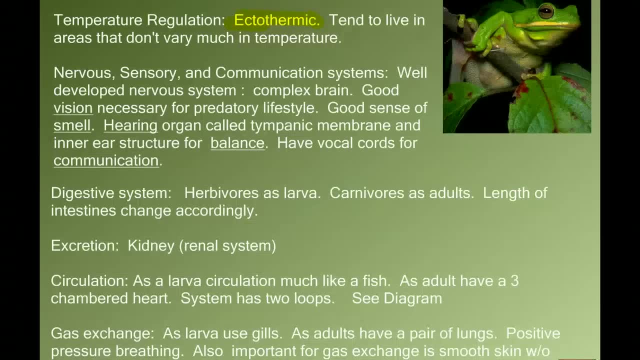 have an external opening, but this membrane can vibrate or pick up vibrations from the air and transmit them to the inner ear structure for hearing, And we know that frogs have vocal cords to vocalize, so vocal communication is very important in frogs. Frogs are predatory. 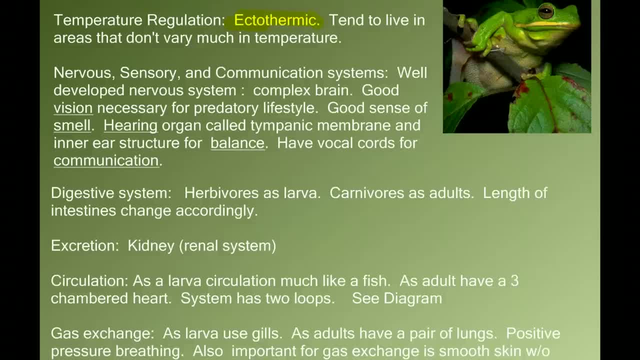 so good eyesight, keen eyesight is important for that type of a lifestyle, One of the more subtle changes that we don't talk about too much, but it's interesting when we look at the digestive system, when their tadpoles, their herbivores, meaning they feed on vegetable. matter, and as adults they're carnivores. they feed on other animals, insects and such, but the herbivores have a longer digestive system. The length of the intestine relative to the overall size of the body is larger in herbivores than it is in carnivors, and 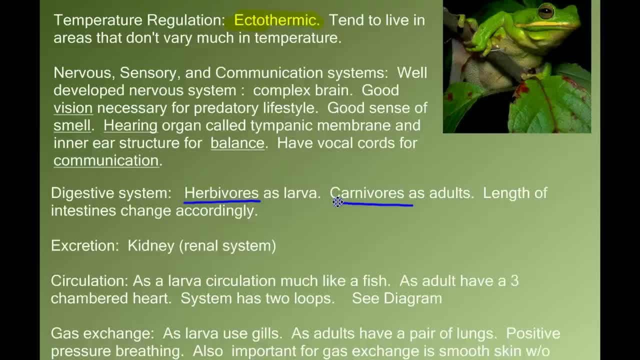 we see this change from the larva to the adult. We're not going to talk too much about the other animals because it's not going to much about the function of the kidney now, but if you think about the job of the kidney to get rid of metabolic waste and also eliminate excess water when we live on land. excess water is not near as much of a problem as not enough water, and so kidneys have to evolve a way to conserve water, and the terrestrial adult versions of the amphibians have to deal with this water conservation issue. so the function of the kidneys to do that it's a very important idea. now we get to. 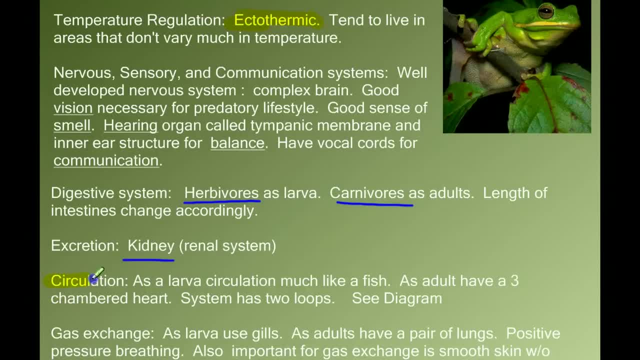 the circulatory system of the amphibians. we have to stop and draw some pictures, but the the circulatory system of the tadpole is much like that of a fish. it's a two chambered heart with a single loop. but in the adult amphibian we have a much different system. we have a three chambered heart. 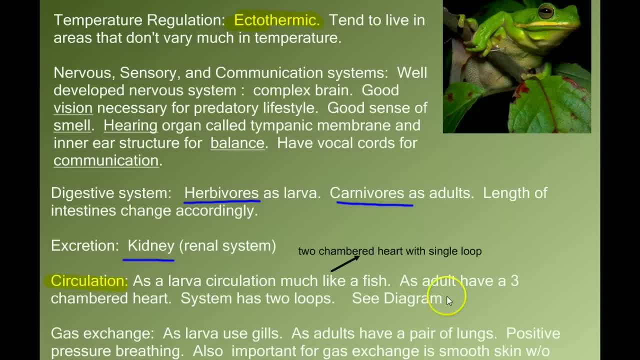 and the system has two loops, which is interesting. so we need to draw a diagram to see why. but think about what's different between the tadpole and the adult. we're going from gills to lungs and in that change from gills to lungs, it alters the shape of the circulatory. 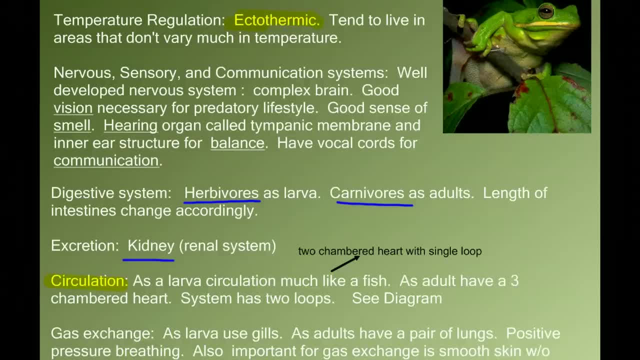 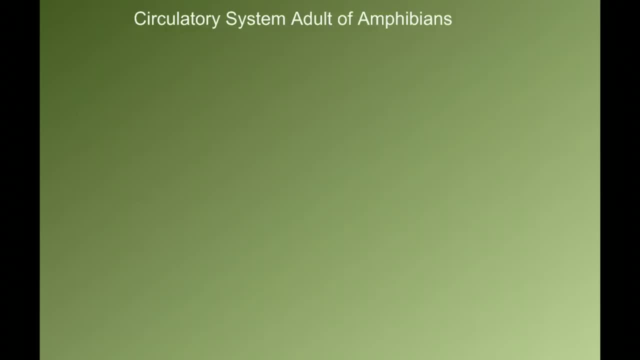 system, because we have to send the blood to the lungs to be oxygenated rather than to the gills. so let's draw some pictures now remember what we're going to draw. here is again a schematic diagram, meaning it's not what it really looks like, but it shows us the parts we need to know. so we'll start off by 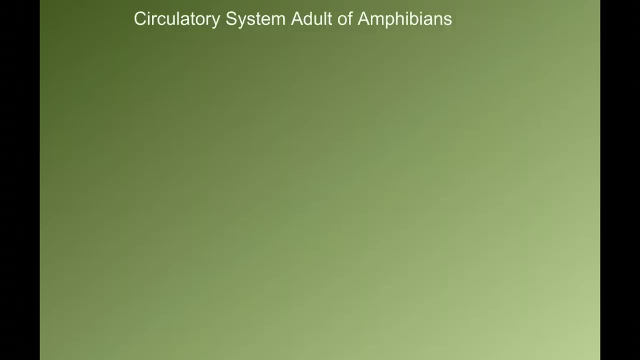 drawing the heart and the amphibian adult amphibian heart is a three chambered heart. so we're gonna draw a structure that looks like this: there's one chamber, here's another chamber and here's the third chamber, and we'll make this at the top, something like this. so there's our three chambered heart. so 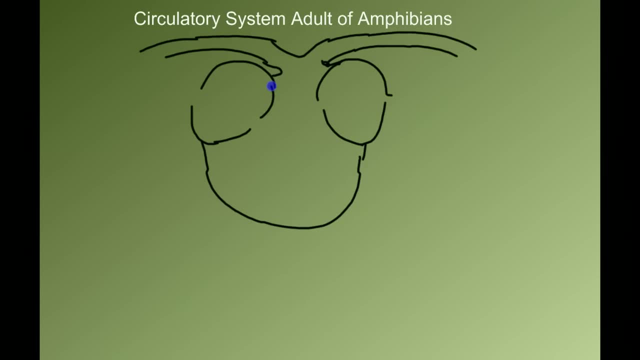 we'll add to this and you'll see it kind of comes together as we move along. but here's our heart and we have three chambers. we have a right atrium and we have a left atrium. now you may be stopping right now saying: mr savage, you got this wrong because you just put the right on left. 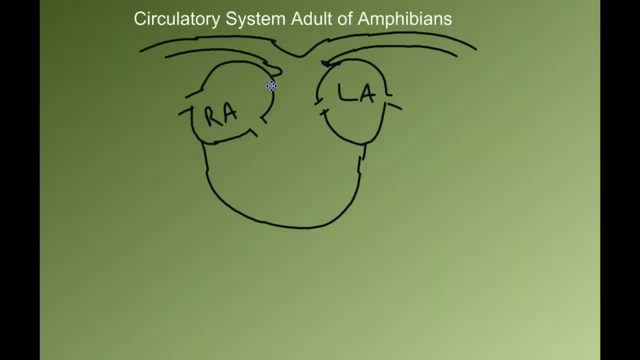 and left on the right, and while I may have a little dyslexia- which is true- we're not looking at it from our perspective. look at it from the perspective of the frog. this side is the frogs right and this side's the frogs left, so I actually have labeled them correctly. 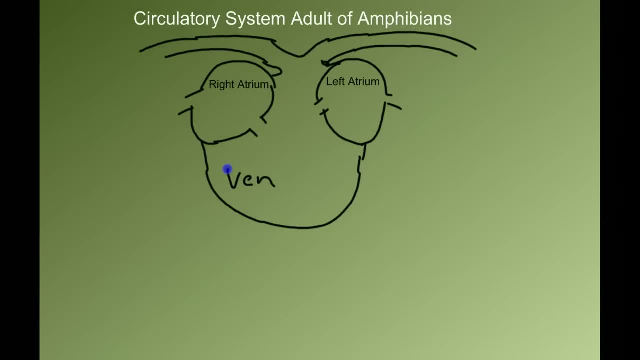 and the third chamber is the ventricle. so we have three chambers, two atria and one ventricle. now, if we remember from our fish video, the atria always receive blood and the ventricle going to send blood on. so we got think about where 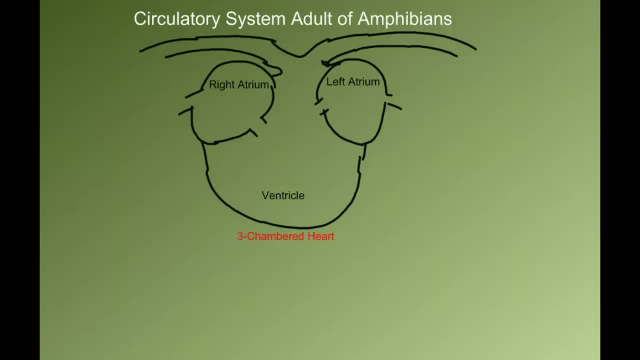 we're receiving blood from, we have to receive and send blood to both the body and the lungs. so let's put the lungs out here and the body out here. when the ventricle compresses, it squeezes blood. whoops, pick this up again. it squeezes blood out to both the lungs and the body. so the 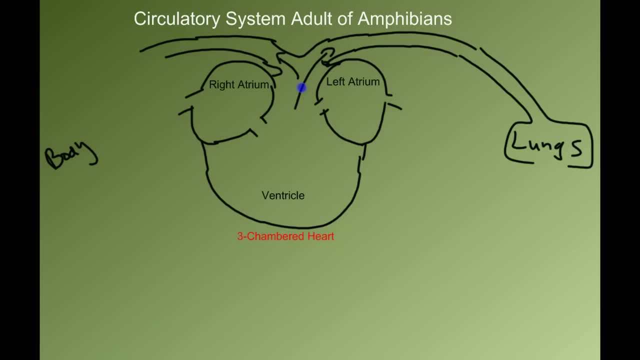 blood comes out to the lungs, where it picks up oxygen and becomes oxygen rich blood, and that blood returns to the heart and what we call the pulmonary loop. the blood that gets pumped out to the body goes out to the body, drops off, oxygenated blood, picks up oxygen, poor blood and returns to the heart. and what? 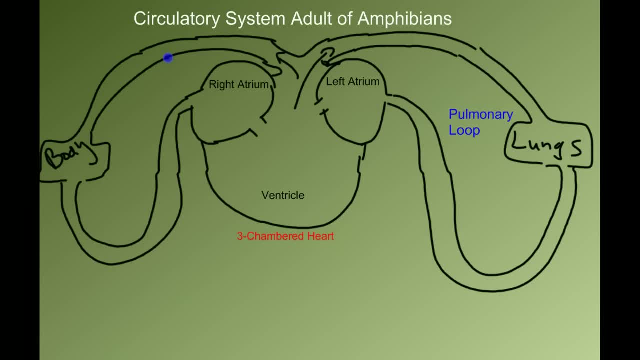 we call the systemic loop because it goes out to the body systems. now let's think about what's good and bad about this system. let's look at where the blood is oxygenated or oxygen rich, and when it's oxygen poor, in the lungs, the blood picks up oxygen. so we're going to draw the oxygen-rich blood in red. 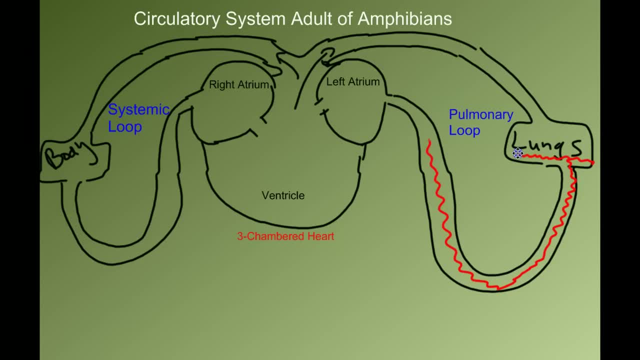 that oxygen-rich blood returns from the lungs into the left atrium. The left atrium then pumps that oxygen-rich blood into the ventricle. The ventricle then compresses and squeezes that oxygen-rich blood out. Now notice that some of the oxygen-rich blood goes right back to the lungs. 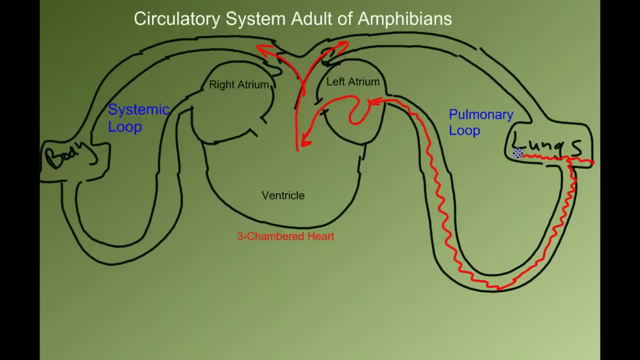 That's a little inefficient- We were just there- But some of that oxygen-rich blood goes out to the body and that's a good thing, because we want to send oxygen out to the body's cells and organs. Now, when the blood comes out to the body, oxygen is used up. 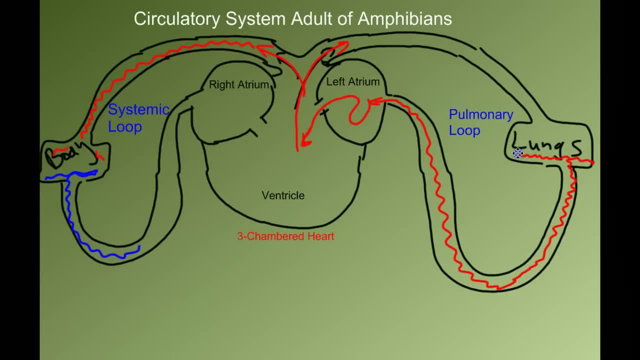 So the blood that comes back from the body is relatively oxygen-poor. So we draw oxygen-poor blood in blue And blood from the body enters into the right atrium. The right atrium pumps that blood into the ventricle and the ventricle pumps that blood out. 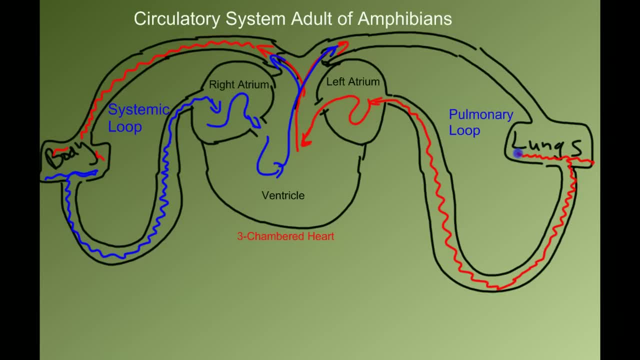 Now notice some of that oxygen-poor. oxygen-poor blood goes back to the body. That's not very efficient- We just came from there- But some of that oxygen-poor blood goes to the lungs, where it gets oxygenated. Now the issue is that in the ventricle 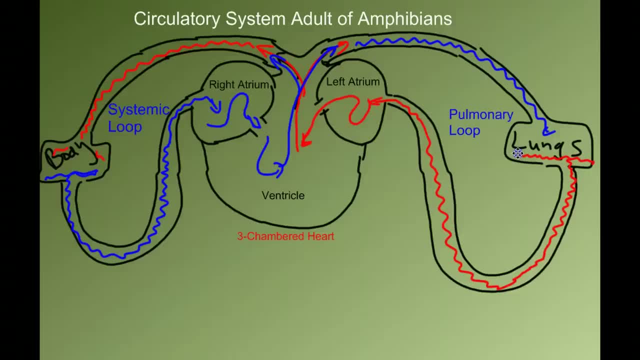 we have this mixing of oxygenated and deoxygenated blood, So that some of the blood going back to the lungs is oxygenated and some of the blood going back out to the body is oxygen-poor. Now it's some kind of a mixture. 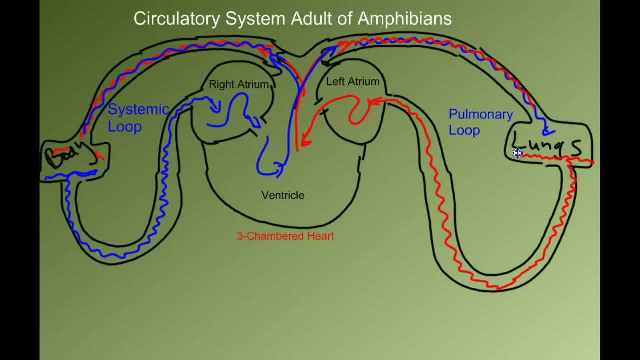 Now, this is not the most efficient system. This is somewhat inefficient, So let's think about this in summary. We have a three-chambered heart and a dual circulation, or two loops. Well, what's going to make up for this inefficiency? 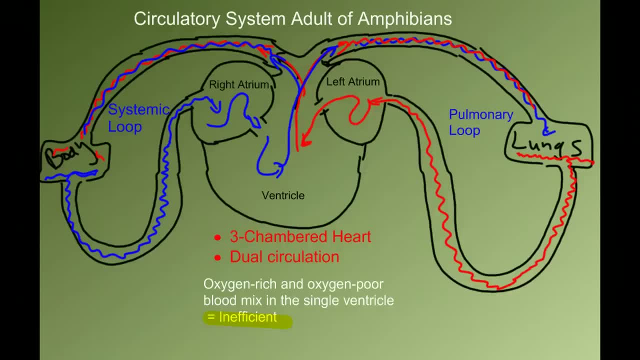 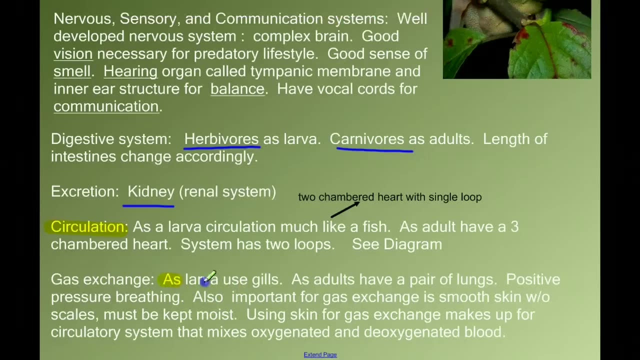 To look to that answer, we need to look at gas exchange. As larva, the amphibians use their gills for gas exchange, But as adults they have a pair of lungs. They engage in what's called positive pressure breathing, And I'll describe that in just a moment. 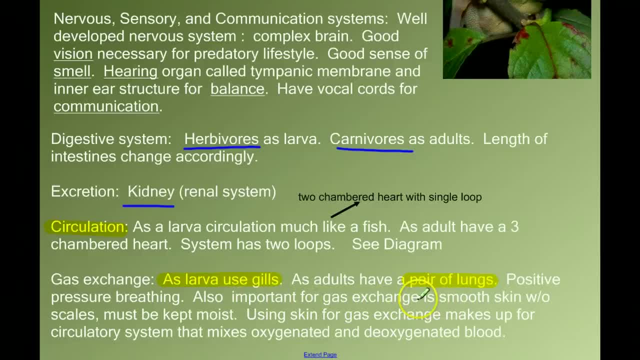 But in addition to their lungs- and this is very important- they have additional gas exchange across their smooth skin, And their skin does not have scales. There are no scales and it must be kept moist. Their skin acts as a secondary gas exchange surface. 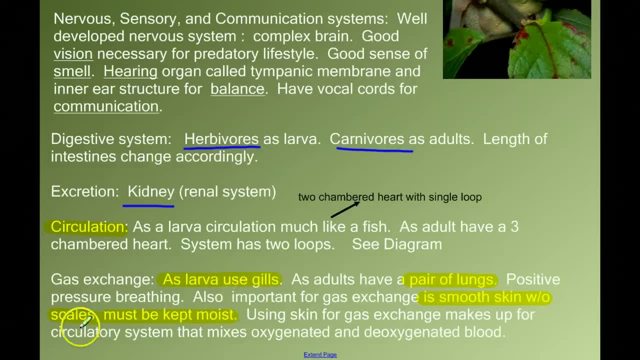 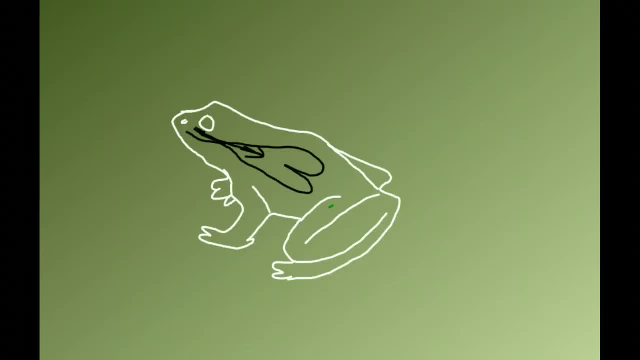 and it makes up for the inefficiency of the circulatory system. Now let's look at this frog. Now I know you're thinking, wow, his art's gotten better. until you see that it's possible that I just traced that. Anyway, here's our frog. 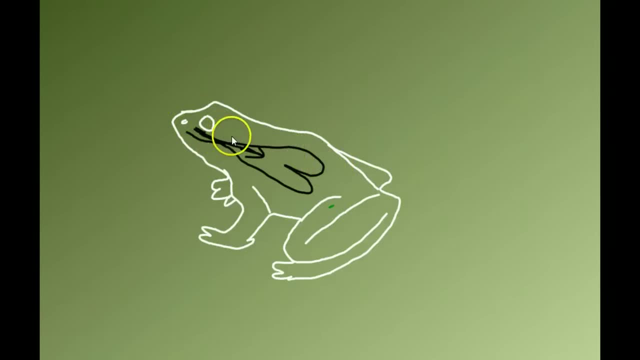 And I've drawn the lungs. It has a pair of lungs, And so the question is: how do you get air down into the lungs? And the answer is called positive pressure breathing. The frogs actually have to push the air down into their lungs. 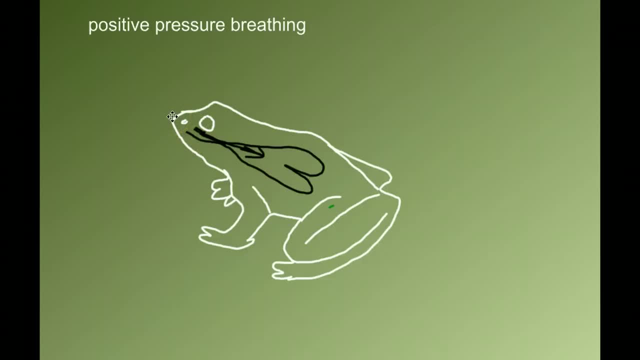 So they open their mouth and open their nostrils and they take a gulp of air. Then they close their nostrils, close their mouth and push the bottom and top of their mouth together and push the air in And these two lungs, like little balloons, inflate. 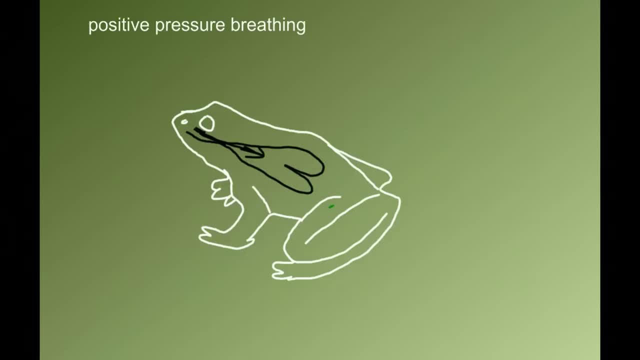 And while they inflate, we exchange gases across the lining of the lungs. They take oxygen in and drop off carbon dioxide, And then when they open their mouth, just like opening the end of the balloon, the air rushes out in a positive push out. 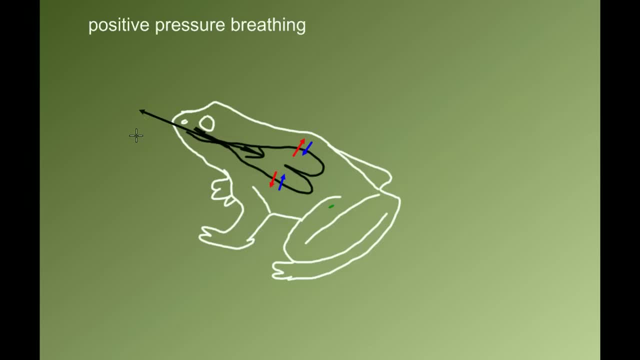 So it's called positive pressure breathing, which is different than the way you breathe, If you think about it. you don't push air down into your lungs, In fact, you pull it from below with a diaphragm, but the amphibians don't have that.